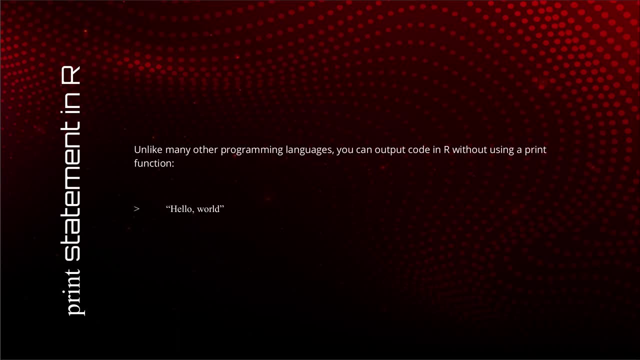 Ok. so if you have used any other programming language, you might have seen that you use a print statement to output text. However, in R, you can simply output text by just writing the text within quotes. It is that simple. However, if you want to, you can use the print. 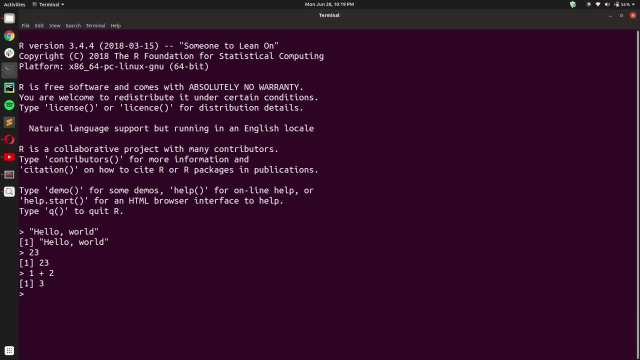 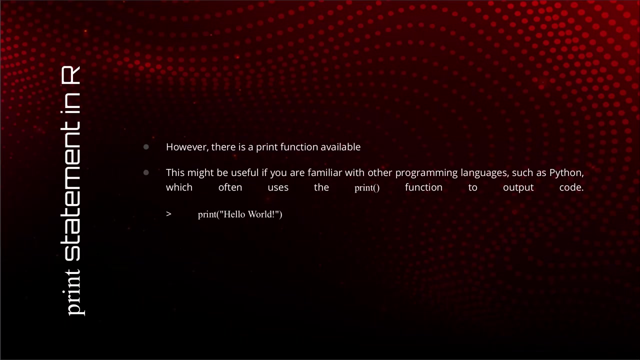 function, but it does not serve much purpose because, like we said, if you want to, you can use the print function Hello world, I get hello world as output, and if I do print hello world, I still get the same output. So why type more verbose when you can get the same result with less characters? 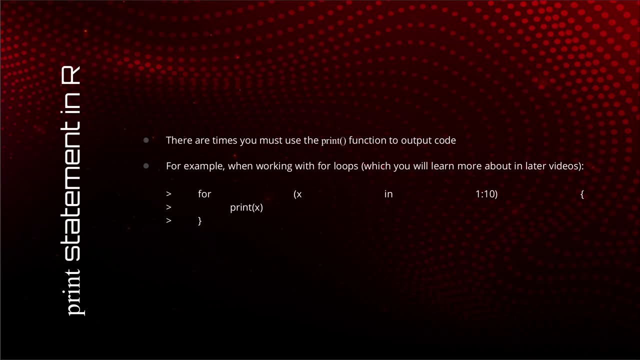 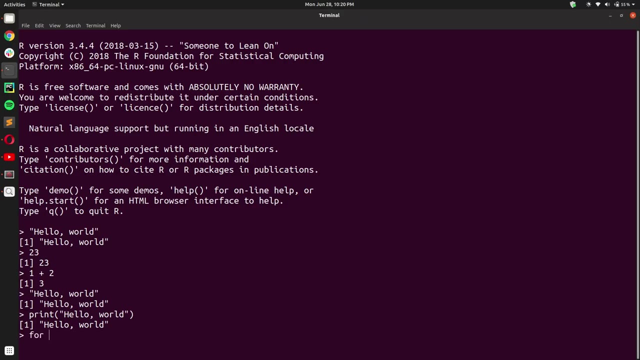 Now there are times that you have to use the print function when there is no other way, And an example of such situation is when you are using a loop and you want to print something inside a loop. Ok, so let us say we have a for loop for x in 1 to 10.. We want to print. 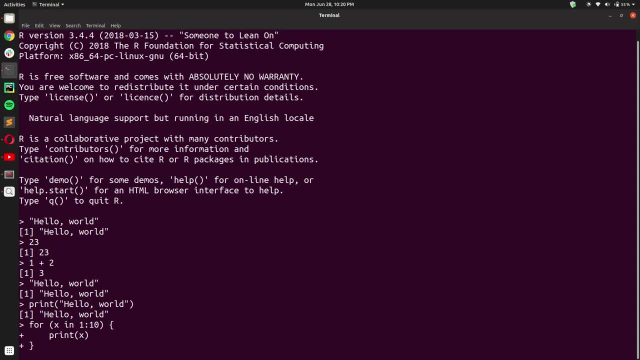 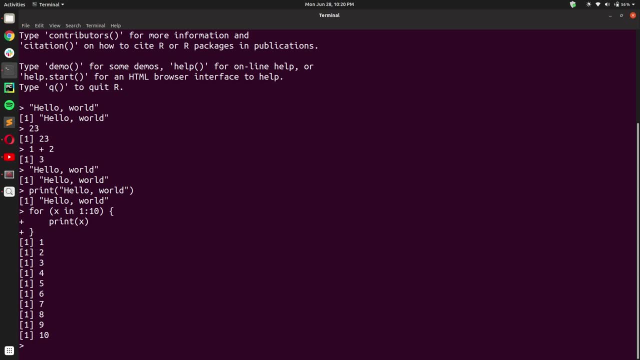 the value of x. Ok, so we got the correct output. The numbers are 1 to 10 at gaps of 1. Which is what we had supplied initially For x in 1 to 10.. 1 colon, 10. it forms a vector. You will learn more about this in the later videos. It forms: 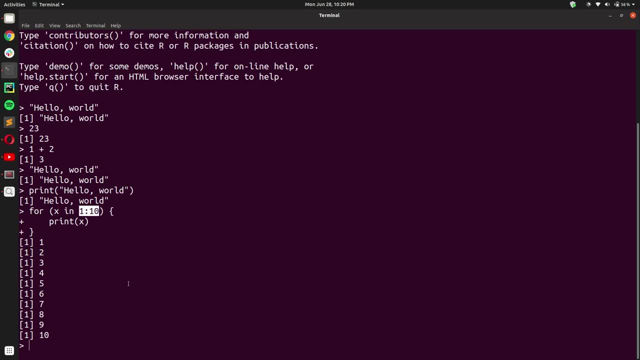 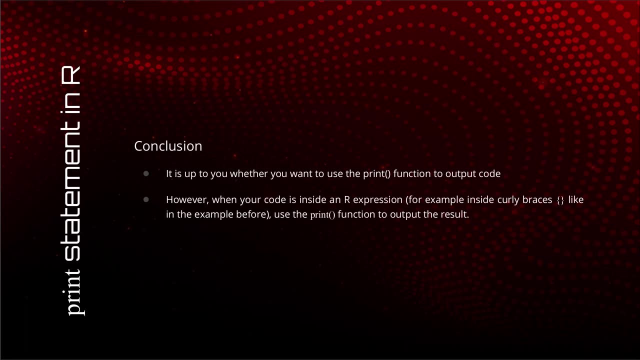 a vector with values spaced 1 apart. So, in conclusion, it is your choice whether you want to use the print function or not. Ok, Ok, Ok, Ok. And the next one, when you want to print something inside of an expression, like we saw with the. 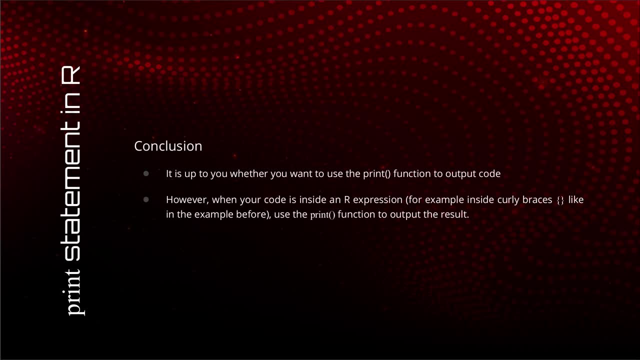 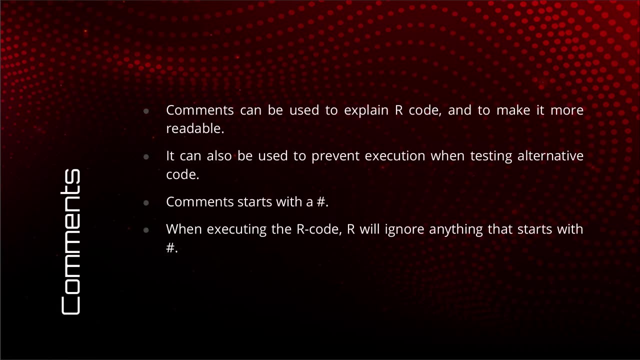 for loop, You have to use the print function. There is no other way. Great, Now that we are done with printing values, let us start talking about comments. What are comments? Comments are something that is used to explain your code and our comments are used to explain. 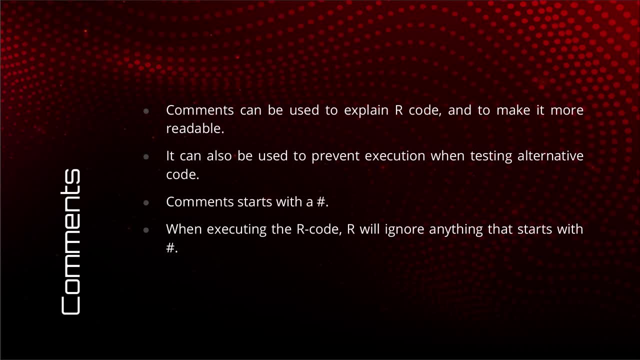 our code. It makes it more readable. Also, sometimes people write their code inside comments and this makes their code non-executable, And this is used when they are testing some alternative code. To write a comment, you simply write your prefix, the line with a hashtag. 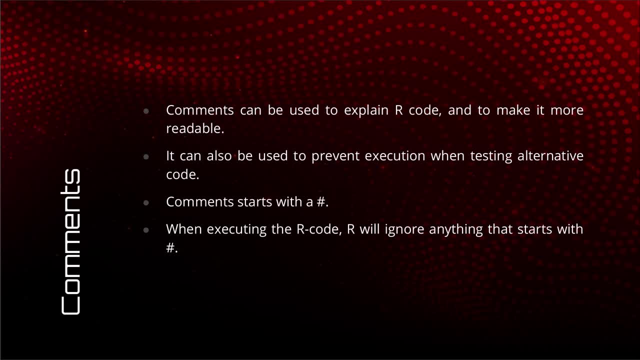 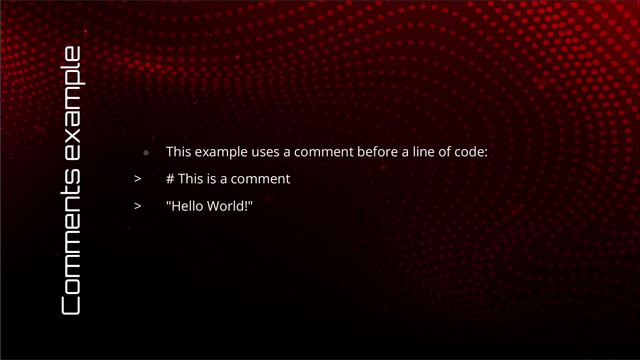 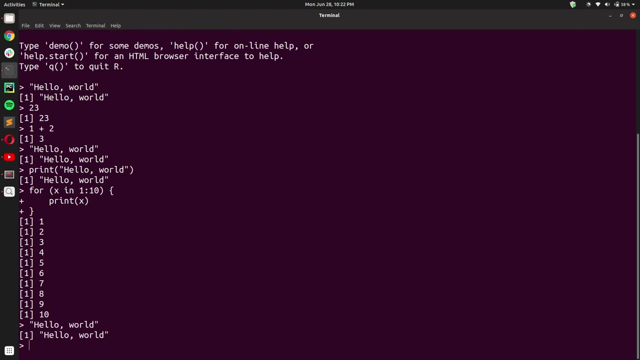 And when you are executing R code, R will ignore anything that starts with the hash mark. Let us see an example. Let us print hello world and write a comment before it. Okay, so as you saw, printing hello world, we get hello world and output. 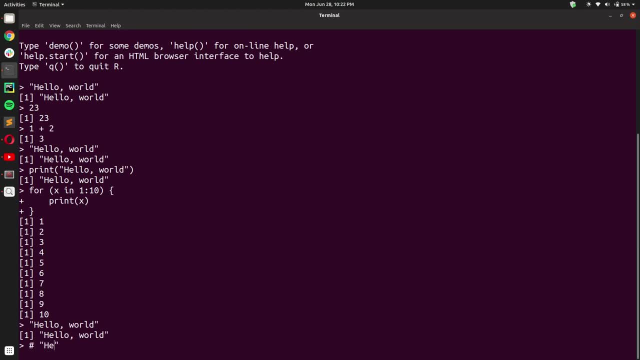 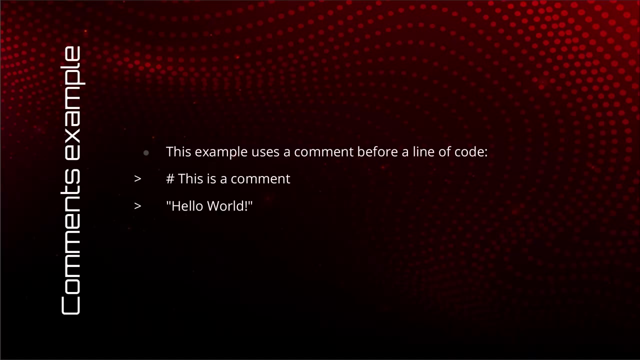 But if we write the same thing but after a hashtag, you will see that I don't get any output. But when I do a simple hello world, I do get output The text I just wrote. Okay, now we we had initially talked about writing a comment on a separate line. 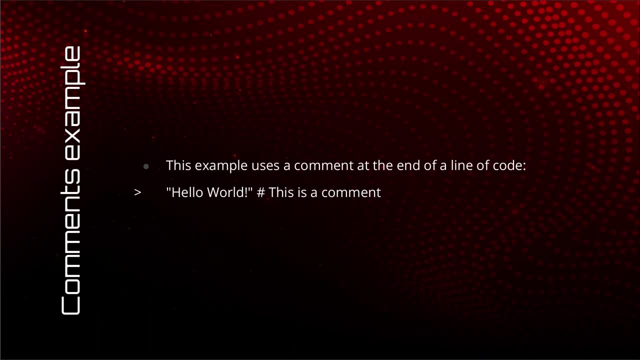 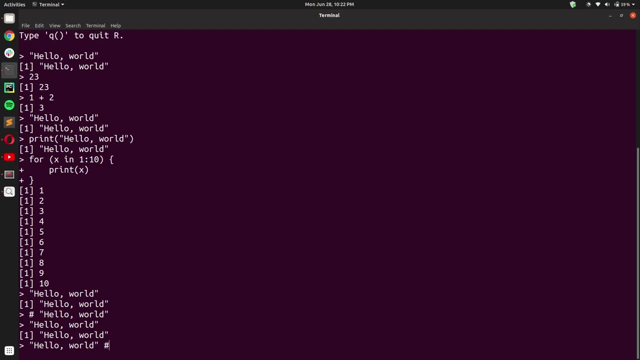 But what if we wanted to write a comment on the same line as code- executable code? You can do that. So, for example, we have the line hello world, which prints hello world, And then we write a comment after the hashtag, And you see that I still get hello world as output, even though I add a comment on. 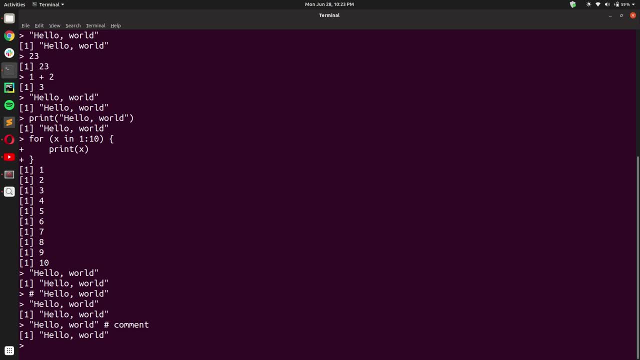 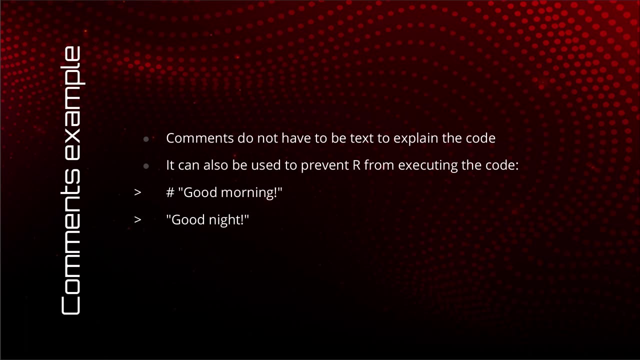 the same line. Anything after the hashtag mark is ignored by the R executor, R interpreter- Great. Like I said before, comments don't always have to explain your code. They can also be used to test alternative code, For example, Hello world. 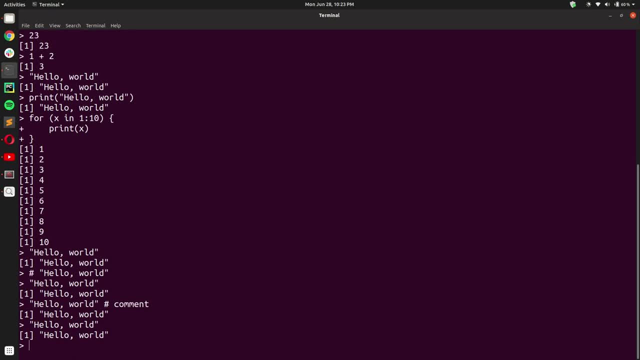 Hello world. Here you are just printing hello world. But what if you wanted to test hello world- not execute it, just test it- but print hello world to, for example? You can do that by writing, by prefixing your code with the hashtag mark. 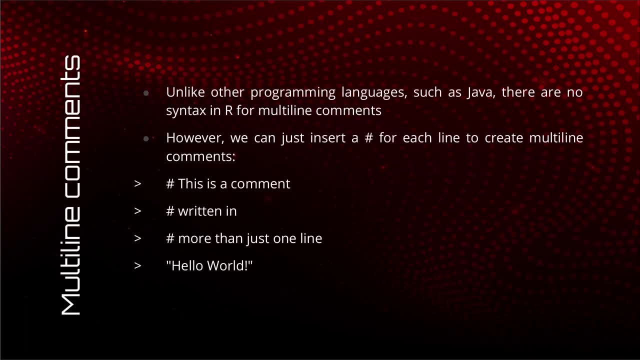 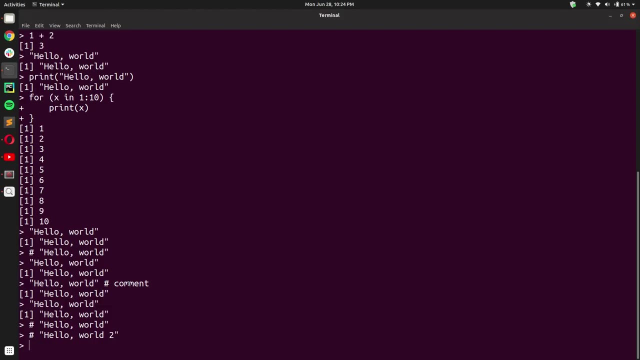 Also, R has multi line commands, but there is no special syntax for multi line commons. You just have to write a hashtag and not execute it. So we can pass that challenge: a hash tag on each line. You have to prefix each line with a hash tag. A simple example: 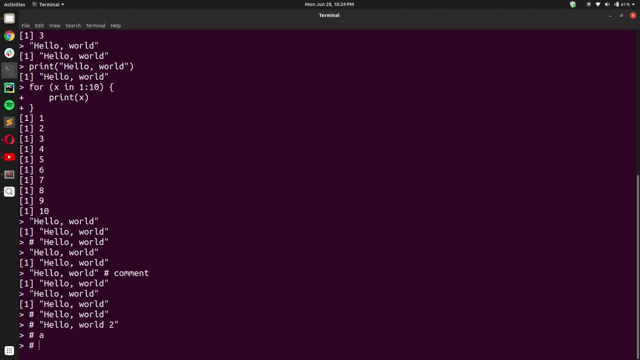 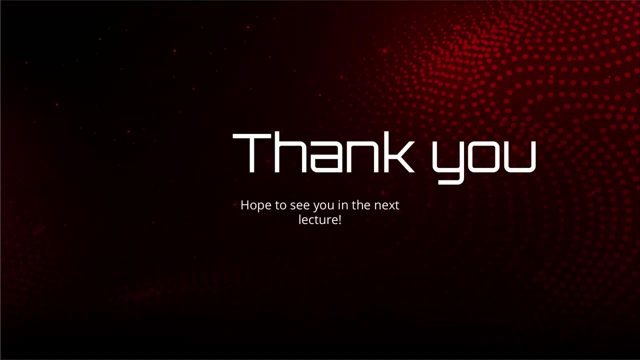 for this is hash tag A, hash tag B, hash tag C and so on. until I just print out D. You have to prefix each line with a hash mark. Okay, I hope you learned something. That was all I had to cover regarding basic R syntax. You now have the necessary tools to tackle. 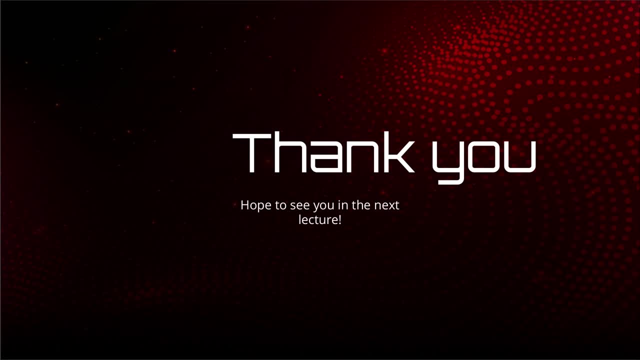 more complex problems and from the next lecture onwards we will start diving deeper into R. See you, Bye. 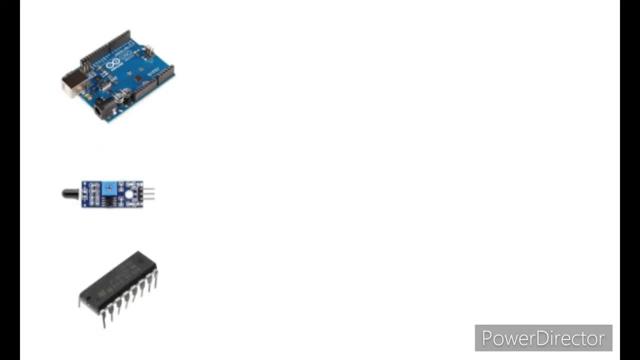 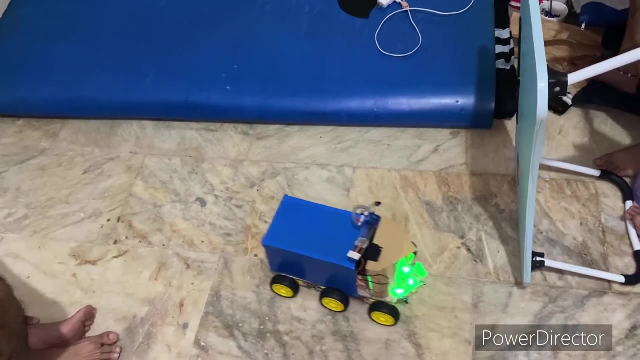 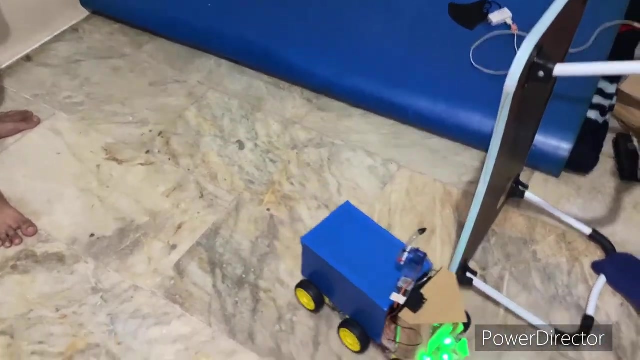 A quick reaction to recognize the little fire can stay away from eccentric harm and misfortunes to humans. In any case, it is hard to distinguish the little fire in the area that is difficult to reach or see by a human. Firefighter Robot is a specialized prototype built to detect 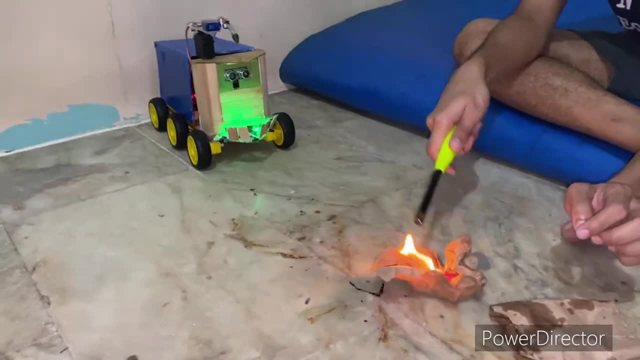 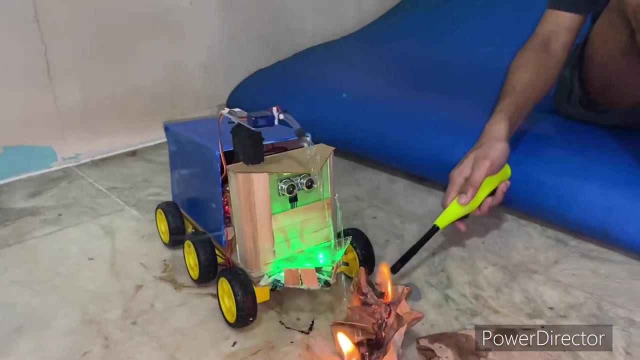 and extinguish fire without taking too much time. The features of the intelligent fireman robot, using fuzzy logic, can detect an obstacle blocking the way and extinguish the fire as soon as possible. Because of this, the tragedies that can cause burning of equipment and being 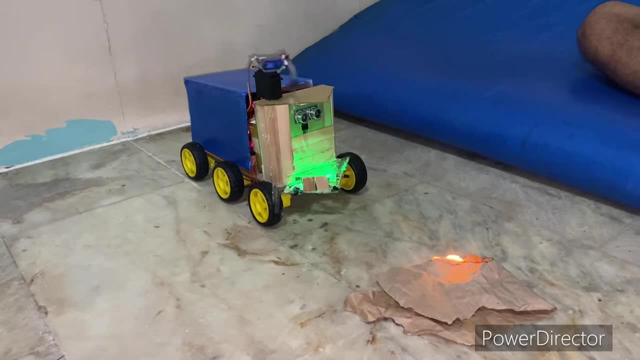 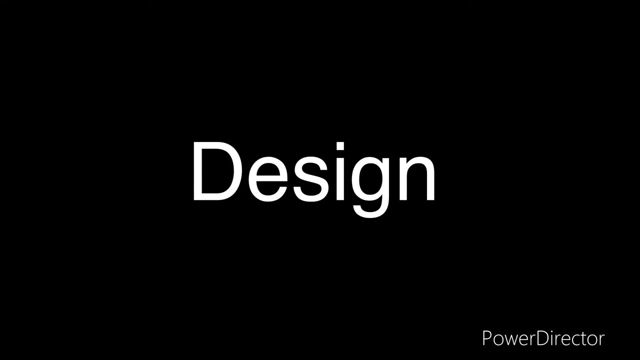 exposed to danger that can hurt people or worse death will be reduced. It has an ultrasonic sensor that can detect an obstacle in front of it and the robot will avoid it so it doesn't crash. It has three flame sensors to precisely determine the location of the fire at the 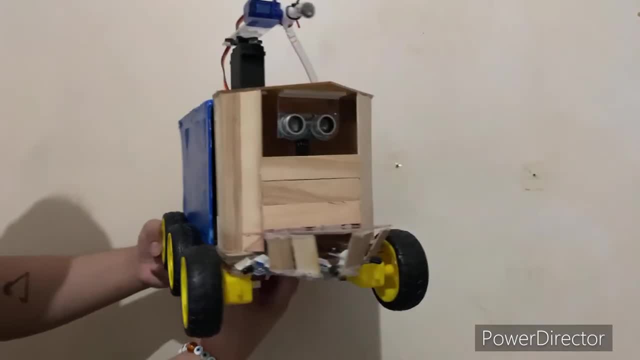 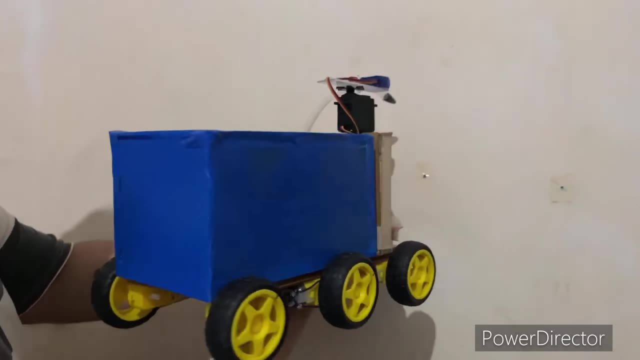 time of fire. Submersible pump for suction and discharge of water at the time of determining the location of the fire. L293IC for activating the wheels to reach the location of the fire. Arduino Uno is the main board we use and it serves as the brain of the prototype Two. 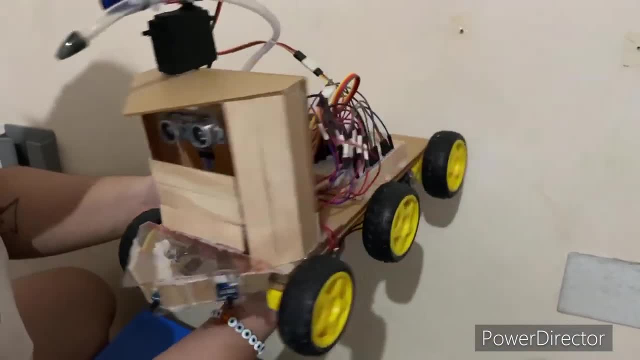 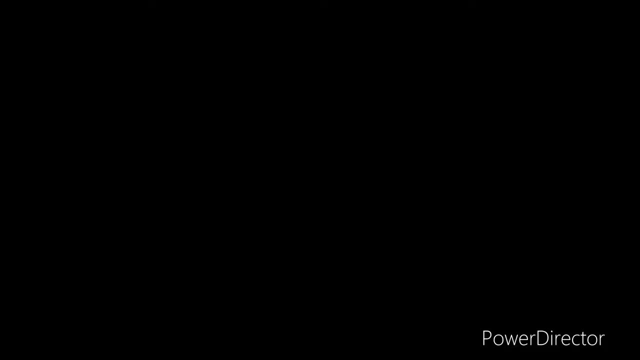 servo motors are used to control the hose that will emit water once a fire is detected. Overall, with the help of our group, the intelligent fireman robot using fuzzy logic was successful in extinguishing the fire, which can be used indoors and in Puppetech.